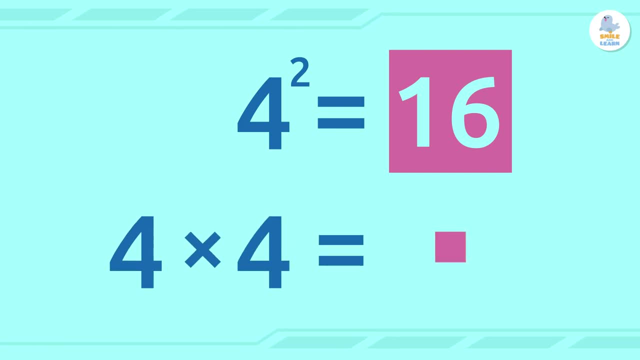 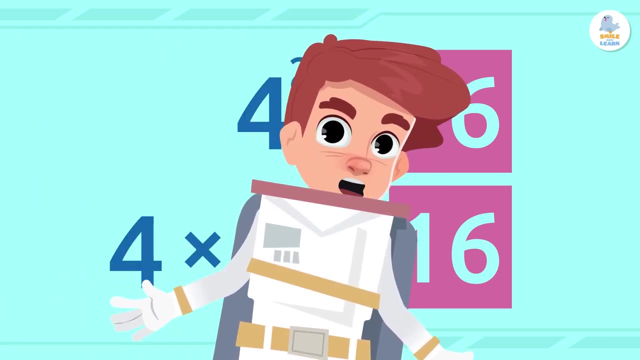 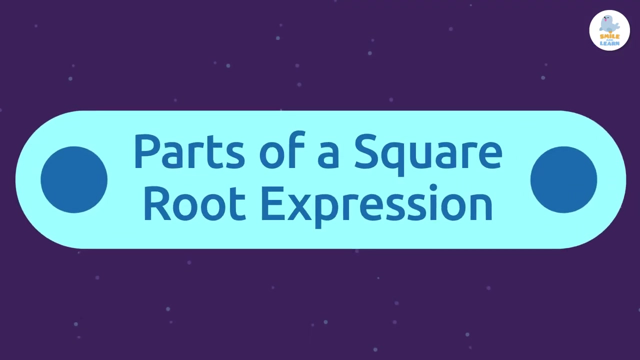 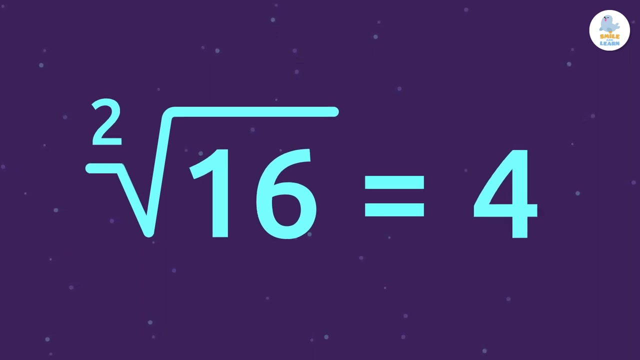 four by itself, or four times four, the product is sixteen Great. This fits perfectly with the definition. But what are the parts of a square root expression? Let's have a look. A square root expression is made up of these parts. The first part: 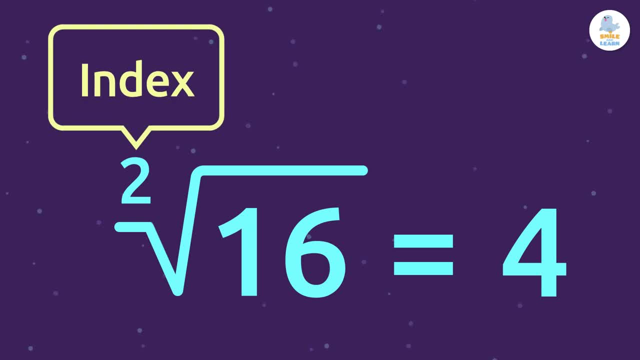 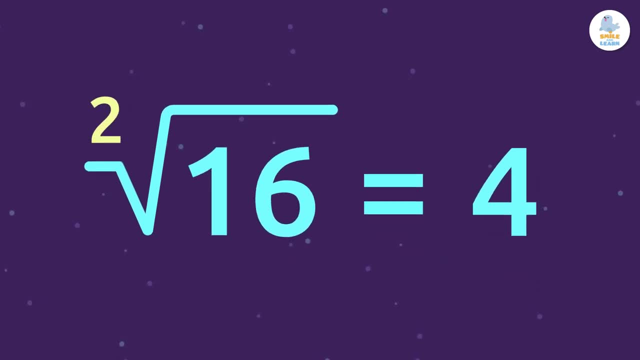 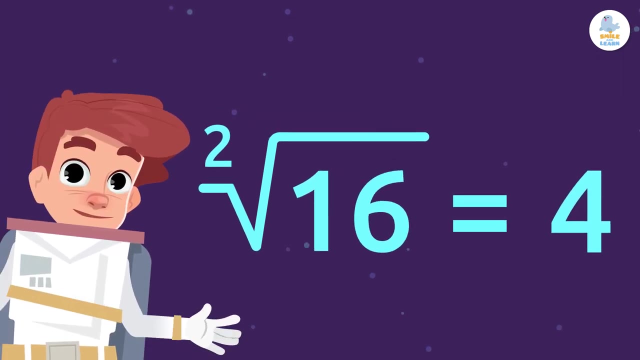 is the index. In our case, we are looking for the square root, so our index is the number two. We can also find other numbers in the index, depending on the type of root it is. For example, if we see a three, it would be a cube root. 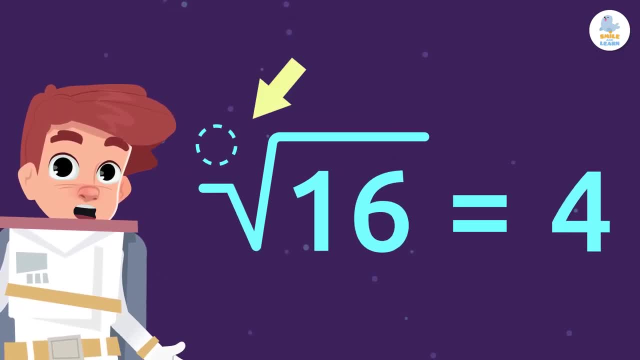 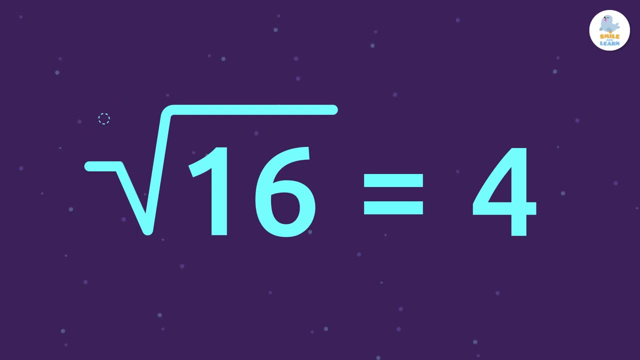 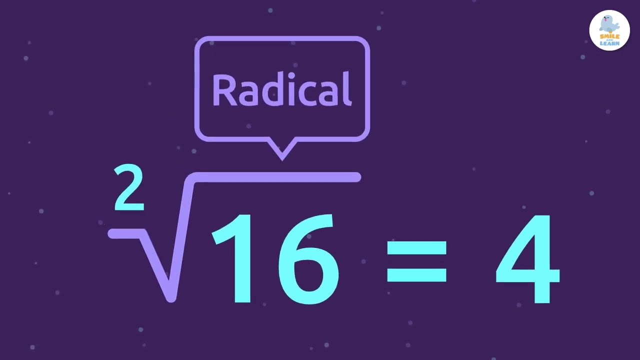 Just so you know, sometimes there is no number where the index goes. If we don't see an index, that always means that it is a square root, so we can just imagine that it has a two as the index. This thing right here that looks like a box is the radical sign, which is what represents. 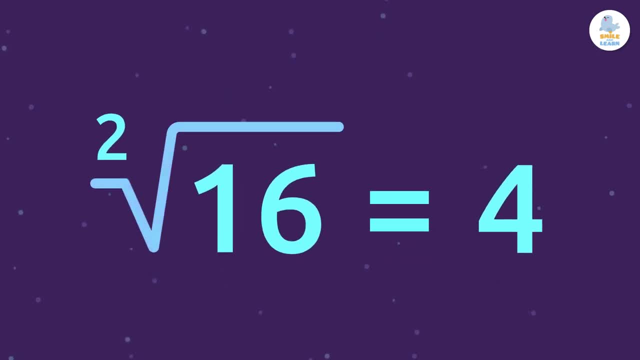 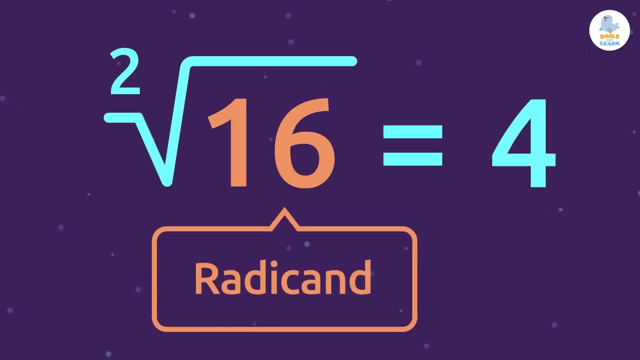 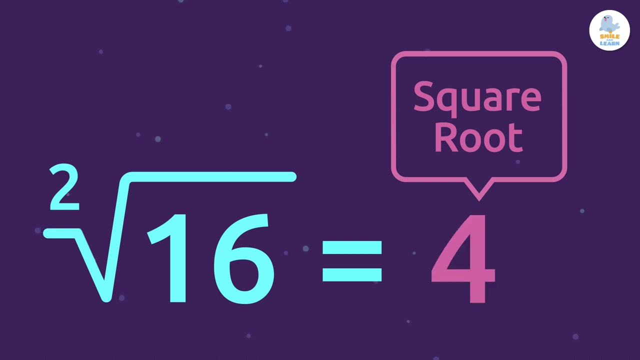 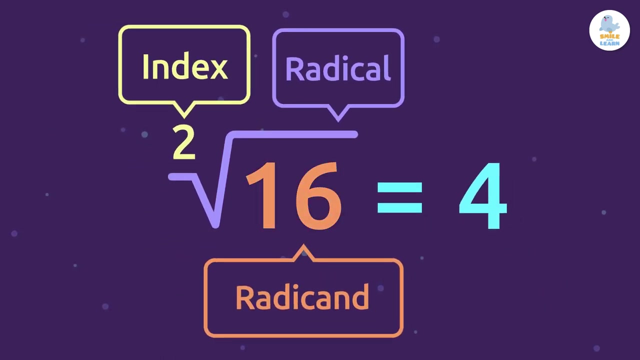 the square root. The number that we see inside the radical sign is called the radicand, which is the number sixteen here. Lastly, the result is called the square root, which in this case is the number four. Great Let's review Index: radical radicand and square root. Good job. 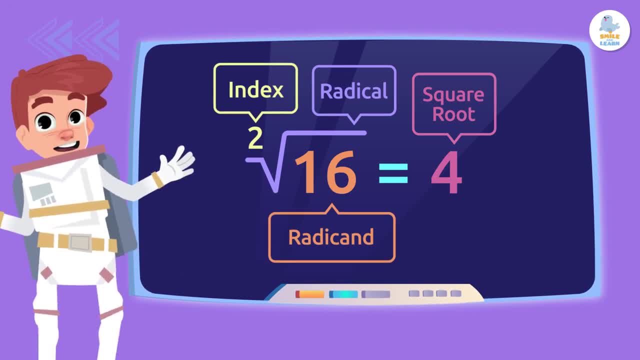 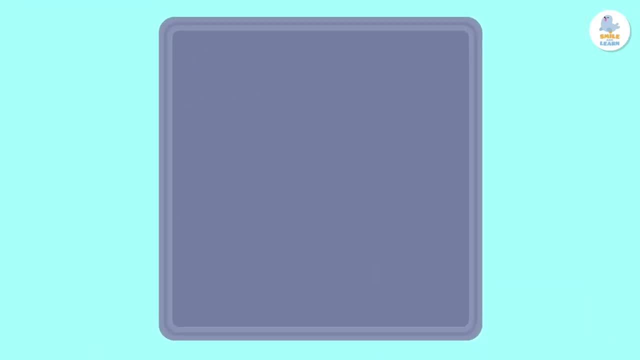 Now that we know what a square root expression is and the parts that make it up, we'll learn what we can do with it. Let's look at an example. Let's look at an example. We have a square tray with twenty-five cakes and we want to know how many cakes are on. 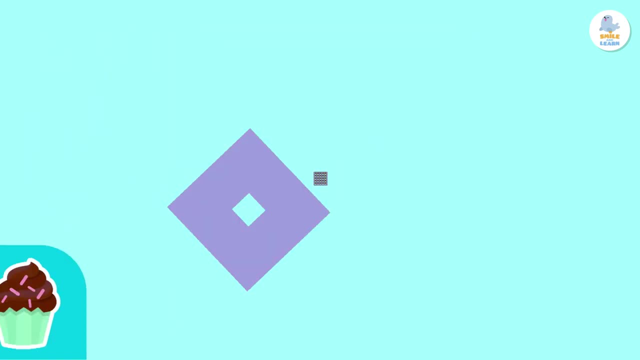 each side. To find out, we have to think of a number that, when multiplied by itself, equals twenty-five. That is, a number squared that results in twenty-five. To calculate this number, we'll take the square root of twenty-five, which is five. 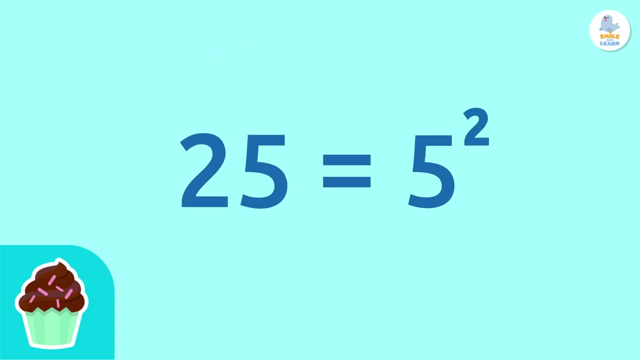 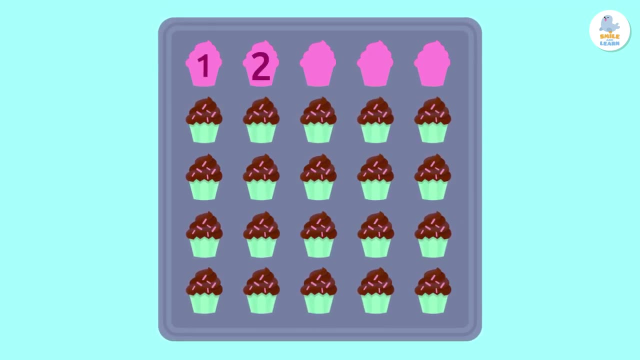 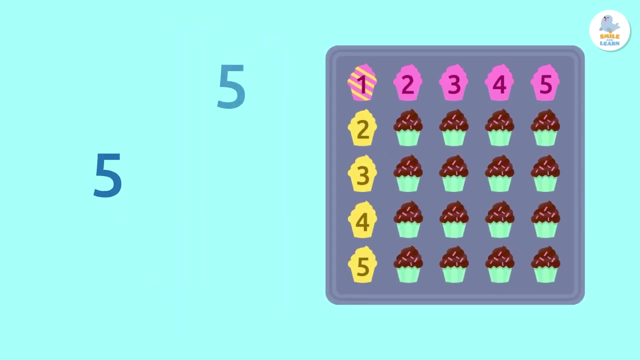 We know this because five squared equals twenty-five. Let's check the result. The horizontal side has one, two, three, four, five columns and the vertical side has one, two, three, four, five rows. As you can see, there are five cakes on each side of the tray. If we square that number, 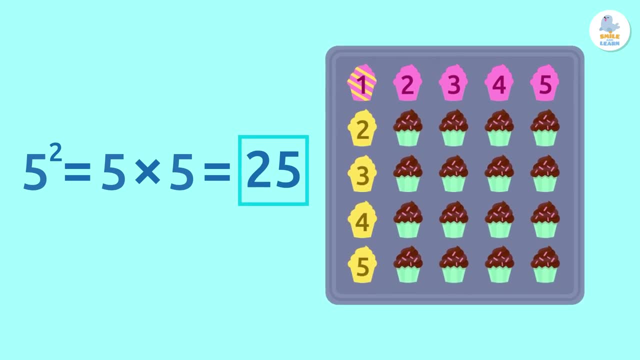 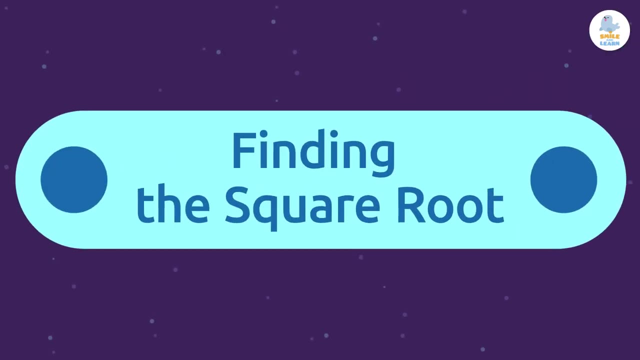 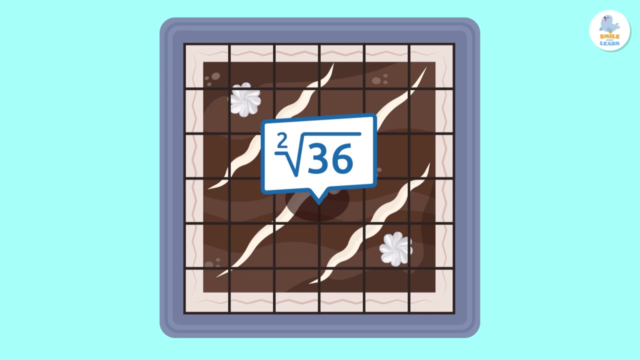 we get a total of twenty-five cakes on the tray. Are you up for finding a square root on your own? Here we have a cake with thirty-six pieces that are all the same size. How many rows and columns does our cake have? Time's up? Do you have an answer? 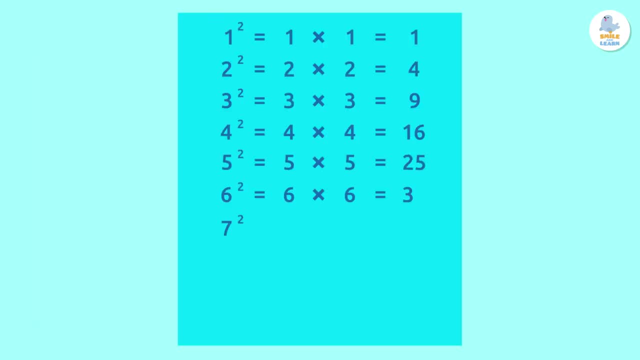 Let's see To know what number squared equals thirty-six. let's have a look at this table. Where is number thirty-six? Hmm, There it is. As you can see, six squared equals thirty-six. This means that six times six equals thirty-six. 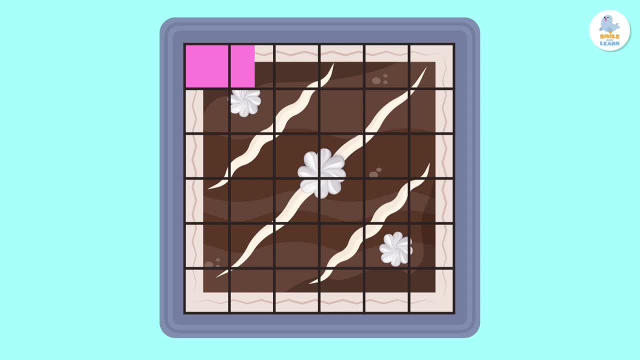 Let's check the result. The horizontal side of our cake has one, two, three, four, five, six columns. Let's check the result. The horizontal side of our cake has one, two, three, four, five, six columns. 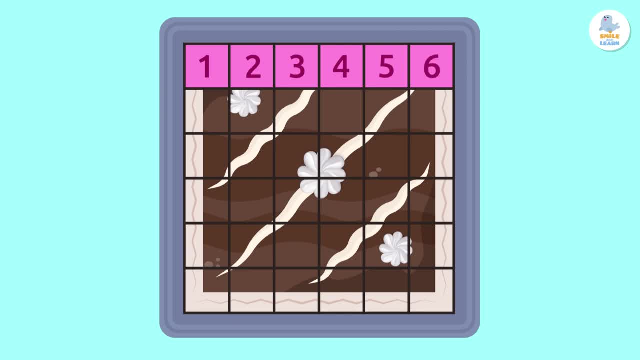 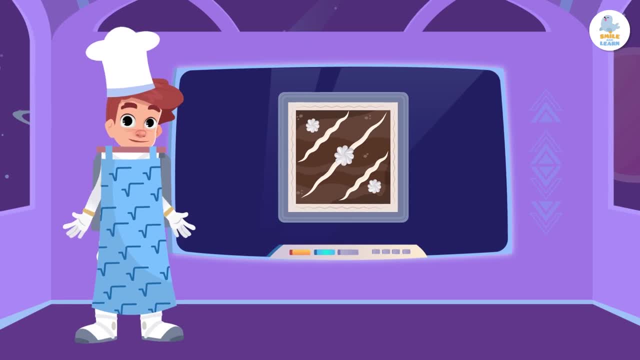 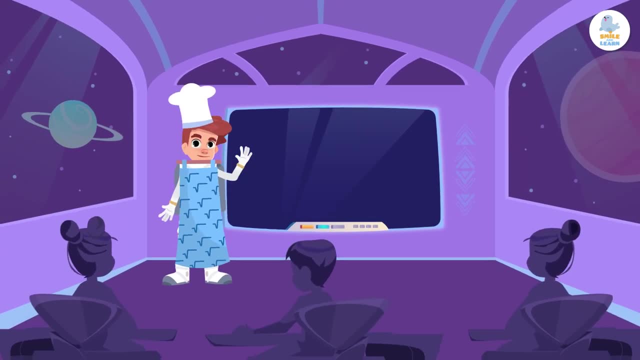 Now we know what a square root is and how to find it. It's snack time. I'm going to have a bit of this delicious chocolate cake. See you soon, friends. This video was made possible by our Patreon supporters. Join the Patreon for free. 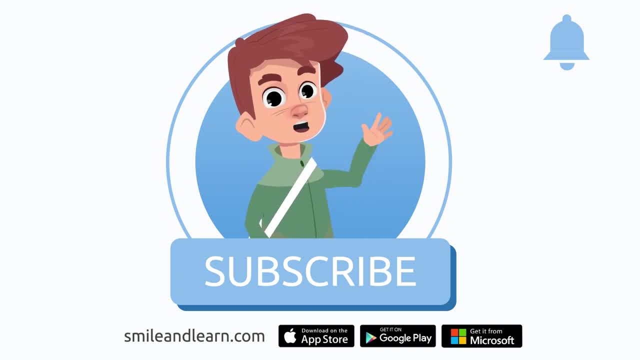 Link in the description. did you know there are many more videos? imagine how much you could learn. subscribe to the smile and learn. educational channel to learn and have fun at the same time.